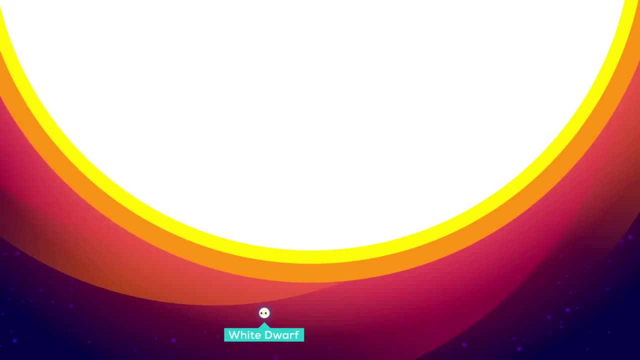 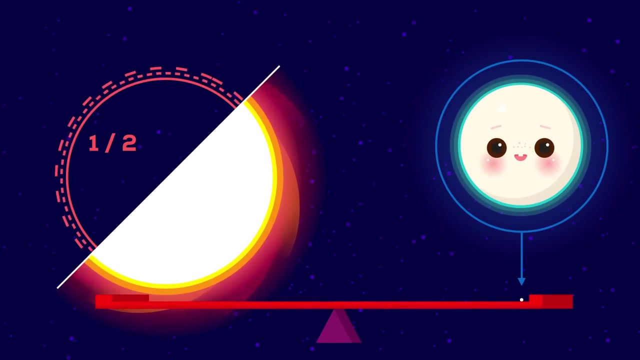 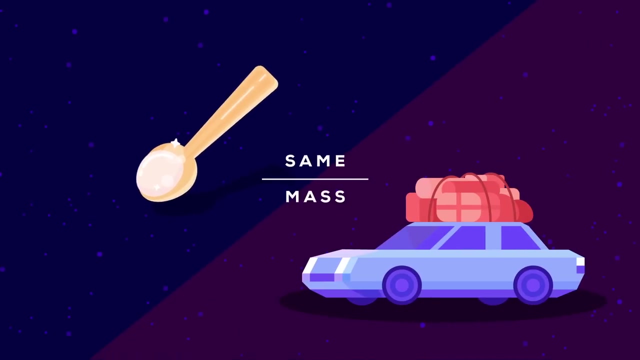 A star corpse. While its former self was about 100 times its diameter, now it's only about as big as Earth, but still with about half of its former mass. This means it's extremely dense. A teaspoon of white dwarf is about as massive as a car. Its surface gravity is over 100,000 times higher than Earth's. If you tried to land on it, you'd immediately be compressed into a steaming puddle. Life around a white dwarf is very unlikely, but possible. Most of them that exist now were former stars that well died. 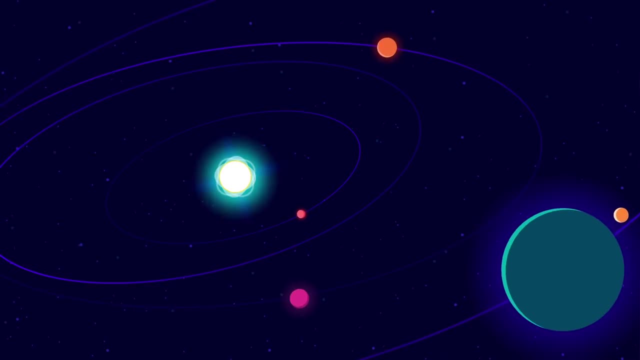 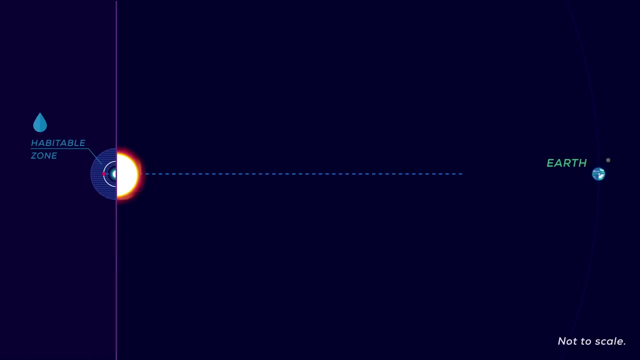 which probably ruined any planets they once had. But that's not all. Since they are so small a planet would need to orbit them about 75 times closer than Earth is to the Sun to have liquid water. This proximity has ups and downsides. 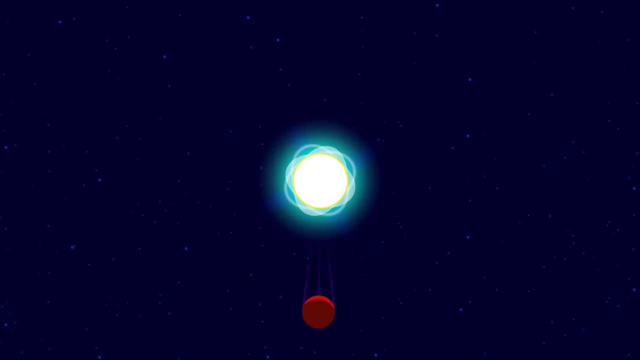 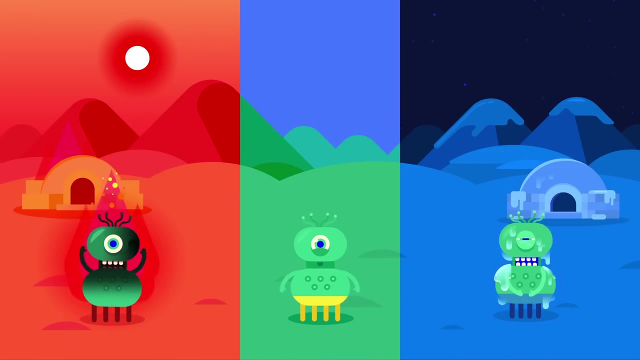 Instead, it would tidily lock the planet, giving it a permanent day and permanent night. At the edges of these day and night zones, life could be possible, But white dwarfs have a very stable energy output, so they might actually be safer to live around than many red dwarfs. 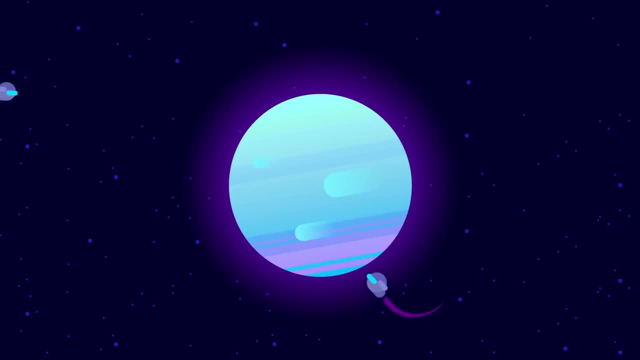 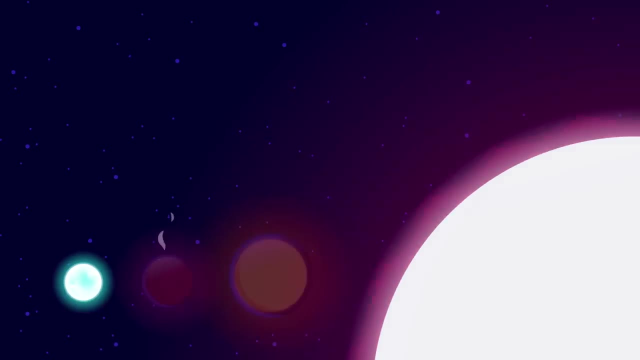 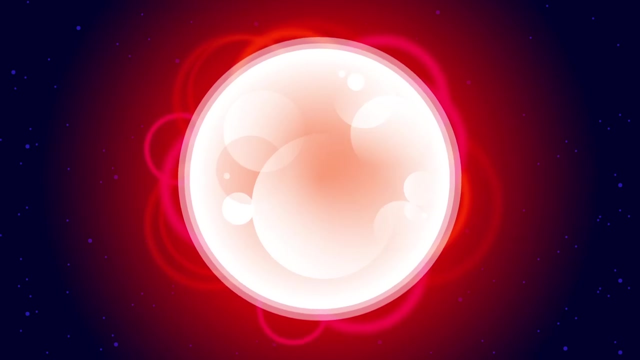 This is still speculation at this point, but if we could find a white dwarf with the right conditions to settle around, we could have a home for many billions of years. But why do they shine so much longer than other star types? White dwarfs are very, very hot, up to 40 times hotter than our Sun. 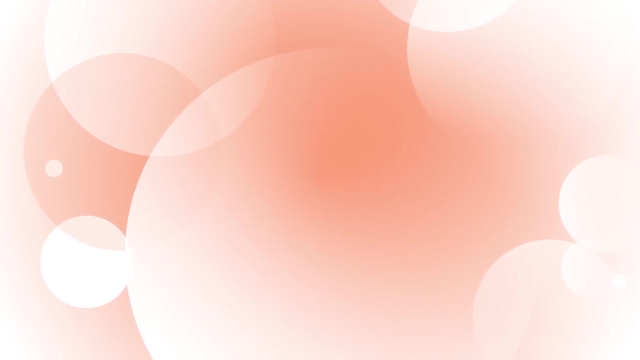 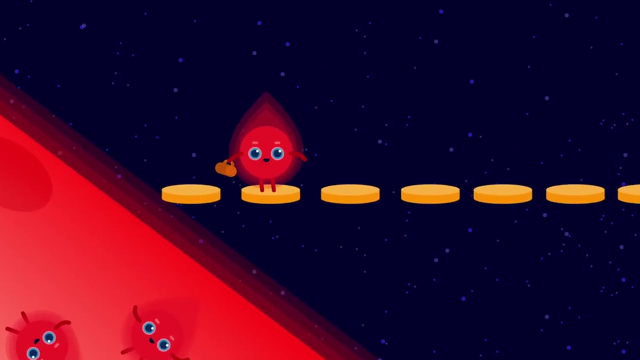 ranking among the hottest objects in the universe, But they are not incredibly active. All the heat inside of them is trapped and has nowhere to go. Only on its outer layer can it escape into space. But space is mostly empty, so heat can't be transferred by conduction. 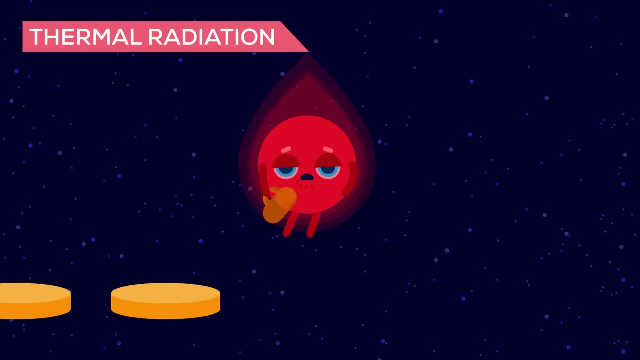 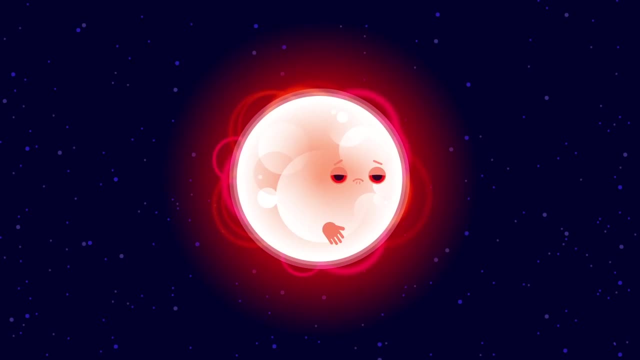 The only way energy can escape is by radiation. This is so inefficient that white dwarfs will take trillions of years to cool down, Which may make them humanity's last refuge. They might be the last sources of light and energy in a dying universe. 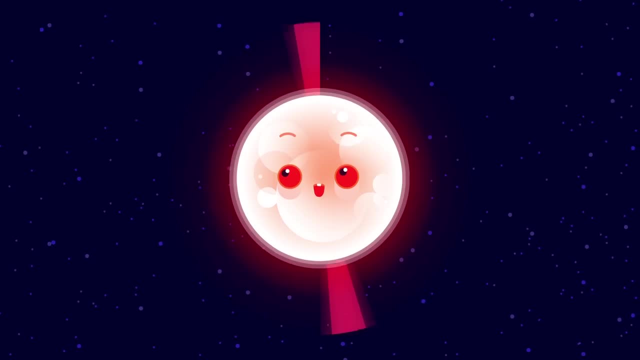 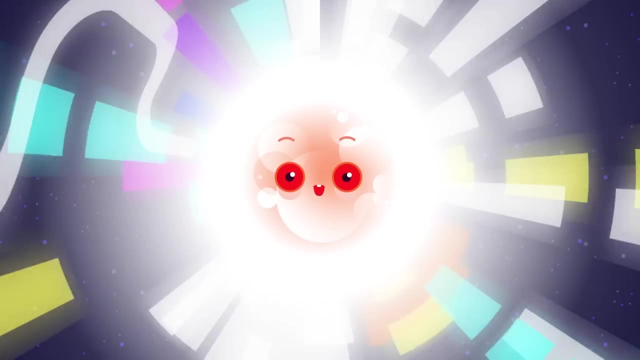 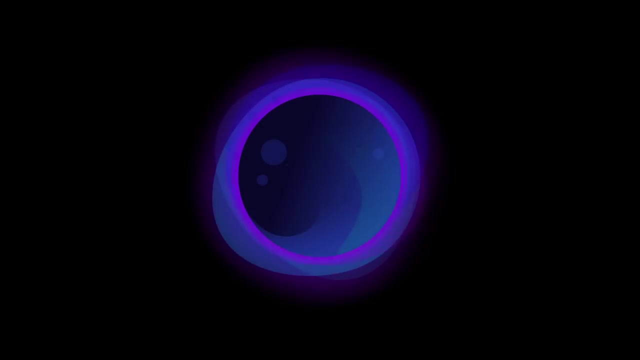 According to some estimates, white dwarfs might shine as long as 100 billion billion years- 10 billion times longer than the universe has existed So far into the future that no regular stars will shine anymore, Galaxies will have evaporated, And only then will the first white dwarf turn into the first black dwarf.